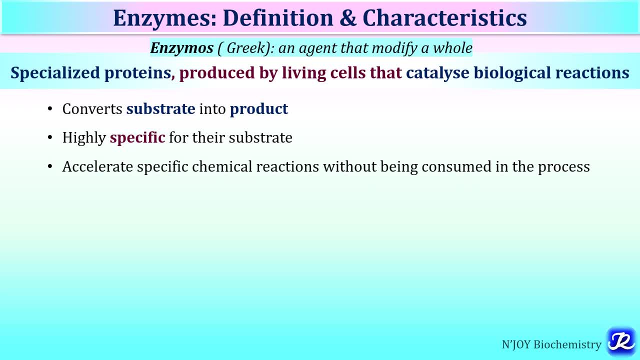 Enzymes are highly specific for their substrate and they accelerate specific chemical reactions without being consumed. in the process, Substrate is a substance on which enzyme acts and by the action of enzyme there is formation of enzyme substrate complex and further there is formation of product. But enzyme is released in this process, which means that enzymes accelerate. 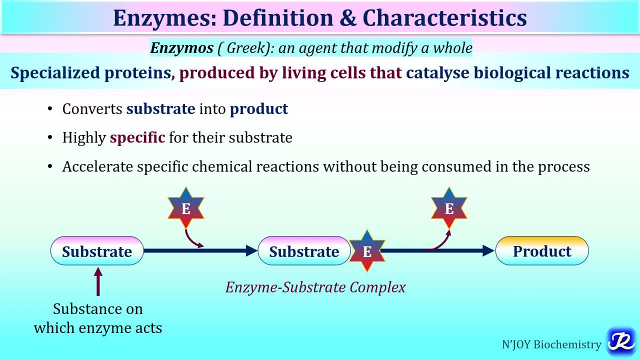 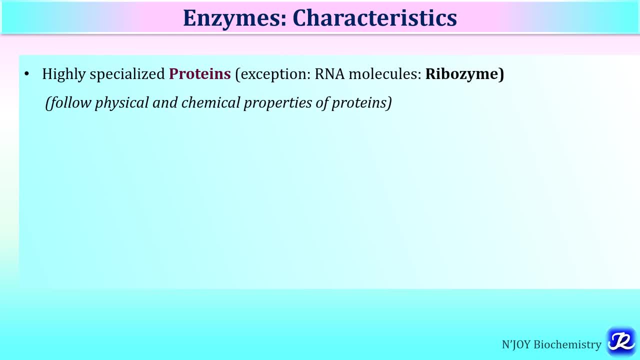 these chemical reactions, but they are not consumed in the process. What are the characteristics of enzymes? Enzymes are highly specialized proteins. Some exceptions are there, for example ribozymes. Enzymes follow physical and chemical properties of proteins. They are heat-lubile. water soluble Enzymes can be precipitated by protein precipitating reagents. 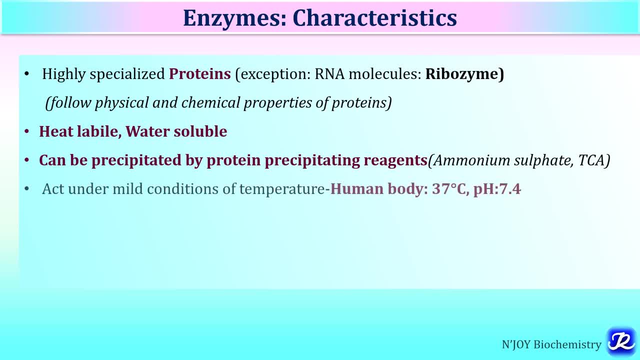 like ammonium sulfate, trichloroacetic acid, Enzymes function under mild conditions of temperature, for example in the human body. enzymes act at optimum temperature of 37 degree centigrade and physiological pH of 7.4.. The catalytic activity of enzyme depends on their native 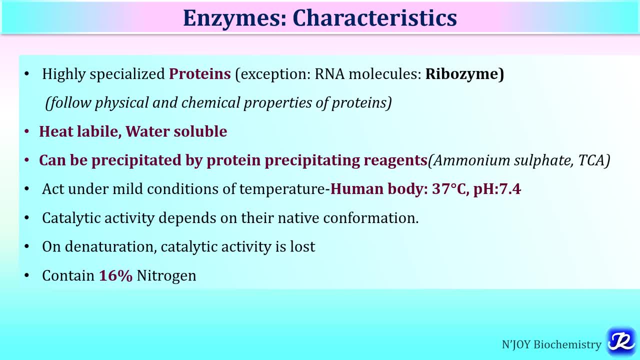 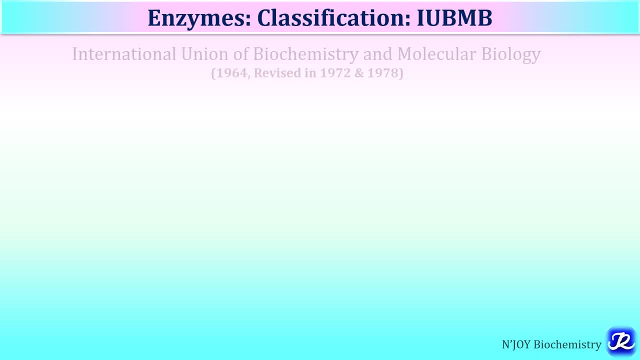 conformation and on denaturation the catalytic activity is lost. Enzymes contain 60% of nitrogen. Enzymes are classified by International Union of Biochemistry and Molecular Biology, which is abbreviated as IUBMB, and the classification of enzyme was done in 1964, which is later. 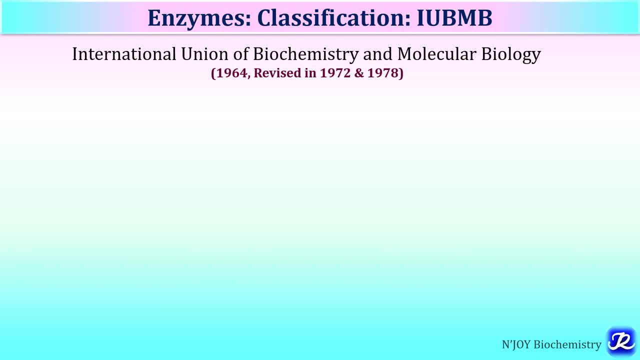 revised in 1972 and 1978.. As for this IUBMB classification, each enzyme has a code number, which is called as enzyme, commission number or EC number, And the EC number has four digits. For example, the hexokinase, it has four digits: 2711. 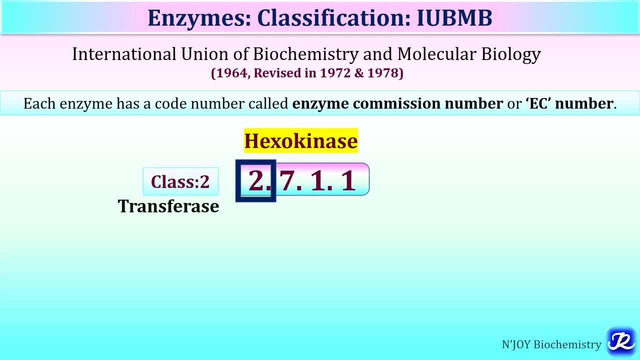 The first digit. it represents the EC2, that is class 2 of enzymes, and class 2 is transferase. So hexokinase belongs to EC2. that is transferase. Second digit here is 7 and it represents subclass. It is the seventh subclass, So this transferases. they have 9 subclasses Out of these 9 subclasses. 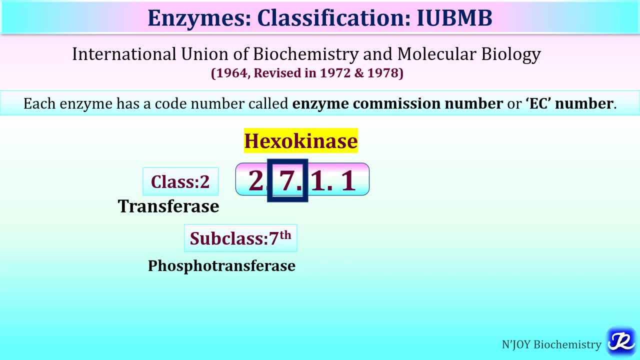 hexokinase belongs to seventh subclass, that is, phosphotransferase. The third digit it represents first sub-subclass, where alcoholic group is the recipient of phosphate group, and the last digit, that is one, it represent the first enzyme, that is, the individual enzyme, hexokinase, which is ATP, hexose phosphotransferase, and this 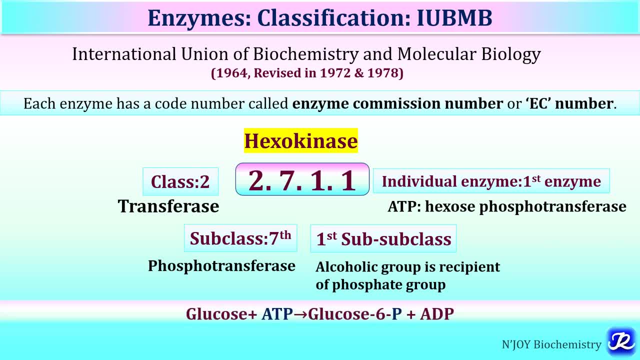 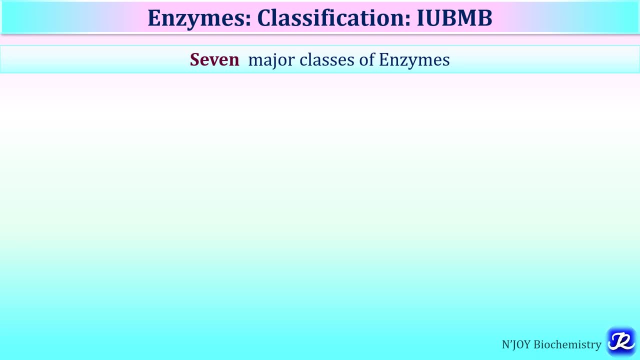 hexokinase, it catalyze the reaction of glycolysis, that is, it transfers phosphate from ATP to glucose, to form glucose 6 phosphate at ADP. According to IUBMB, the enzymes are classified into seven major classes, and these seven classes should be enumerated sequentially. 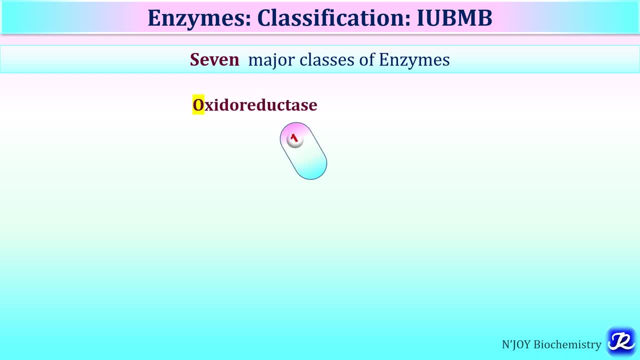 right from the EC1 to EC7. So EC1 includes oxidoreductases. so the first class of enzyme is oxidoreductases. Second class that is EC2, transferases, EC3, hydrolyses, EC4, lyases, EC5, isomerases, EC6. 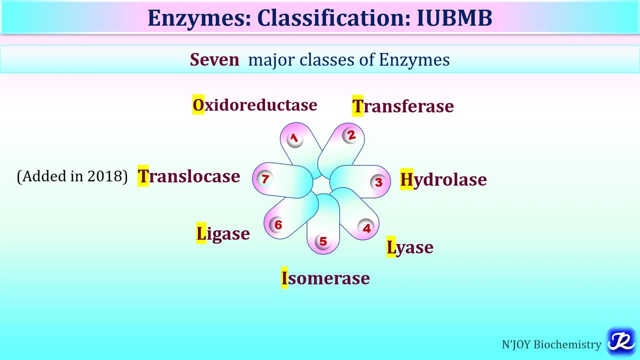 ligases, EC7, translocases, and this has been recently introduced, in 2018.. So there are seven major classes of enzyme, right from the oxidoreductases to translocases, which should be enumerated sequentially. So these are the seven major classes of enzyme, right from the 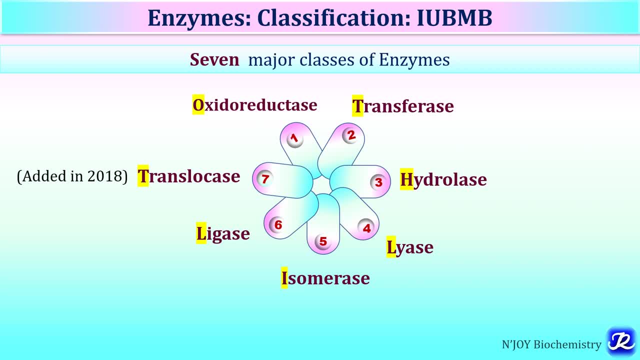 oxidoreductases to translocases, which should be enumerated sequentially from EC1 to EC7, and this can be remembered by mnemonic OTHLYL-T. O stands for oxidoreductases, T for transferases, H for hydrolyses, L for lyases, then isomerases, ligases and, lastly, translocases. Now let's 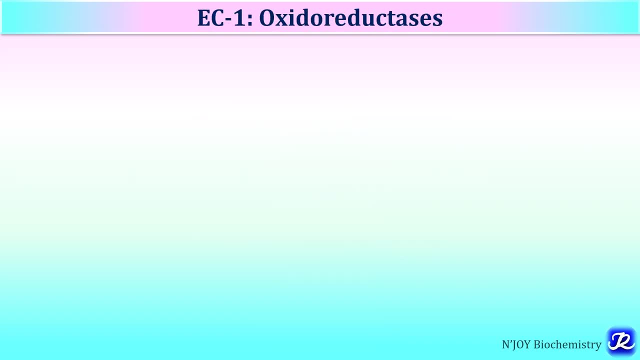 learn about each class and their example. So EC1: it includes oxidoreductases which catalyze oxidation reduction reactions. So this is the first class of enzyme right from the oxidoreductases. Oxidation is removal or loss of hydrogen or loss of electrons, and reduction is gain of hydrogen or 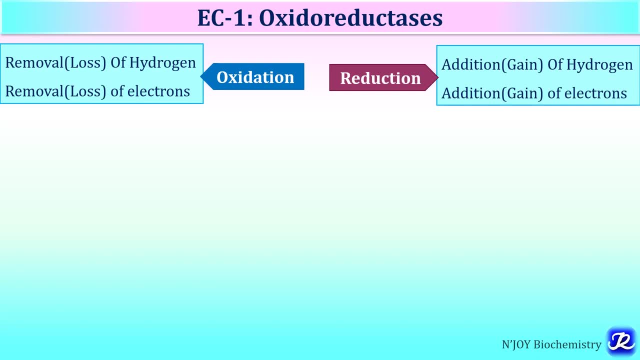 gain of electrons. So these oxidoreductases are the enzyme which catalyze the reactions of biological oxidation. So the reactions can be represented as AH2 plus B, which leads to formation of A plus BH2.. So there is transfer of hydrogen here. there is loss of hydrogen. 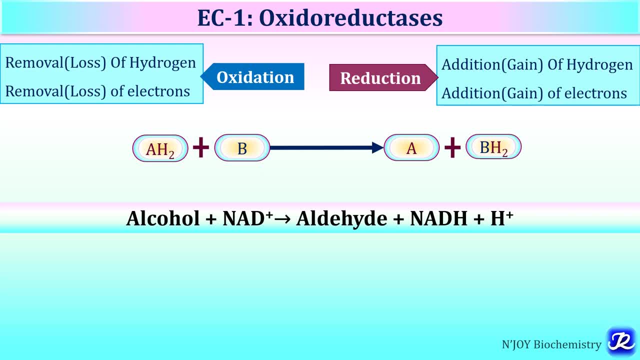 here. So the example is alcohol plus NAD and there is formation of aldehyde plus NADH plus H plus ions. So the hydrogen is transferred from alcohol to the coenzyme NAD to form NADH and there is formation of aldehyde. So there are various examples of oxidoreductases and this reaction is catalyzed. 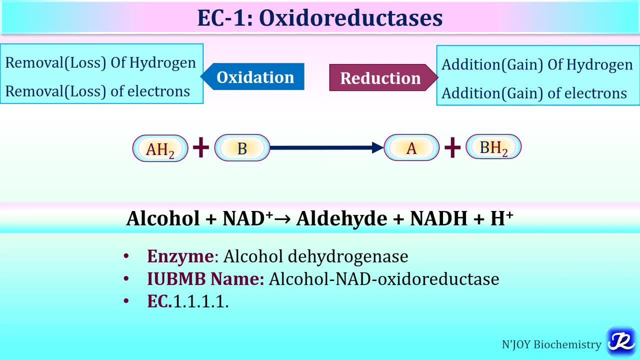 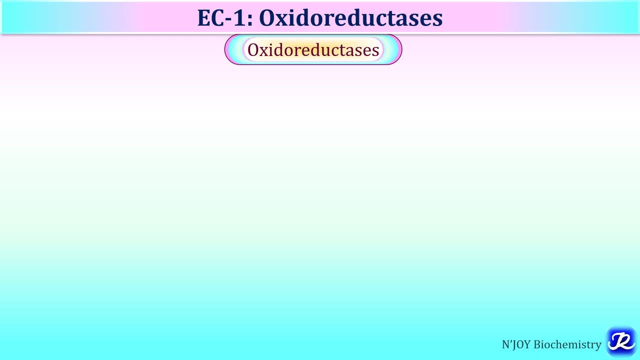 by the enzyme alcohol dehydrogenases, So there is removal of hydrogen. The I OBMB name is alcohol NAD oxidoreductase and the EC number is 1111.. There are various types of oxidoreductases and this has been already explained in video. 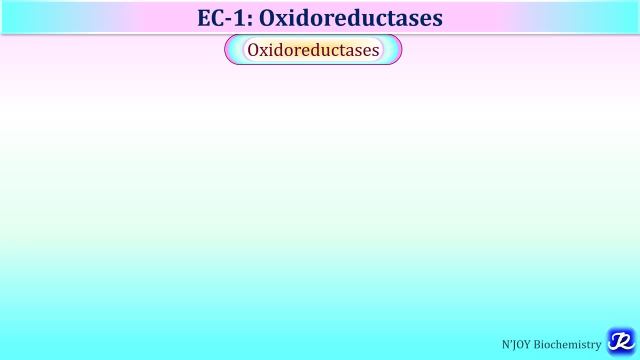 on enzymes of biological oxidation and I am giving the link in the description. So the oxidoreductases can be dehydrogenases which catalyze the removal of hydrogen from substrate. Dehydrogenase can be aerobic dehydrogenase. Dehydrogenase can be acidic dehydrogenase and 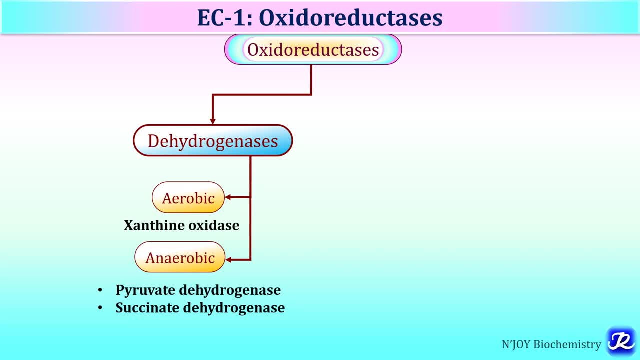 or anaerobic. If oxygen is the hydrogen acceptor, then they are aerobic dehydrogenases, for example xanthine oxidase. They require coenzymes as hydrogen acceptor, like NAD+, NADP+, FMN, FAD. 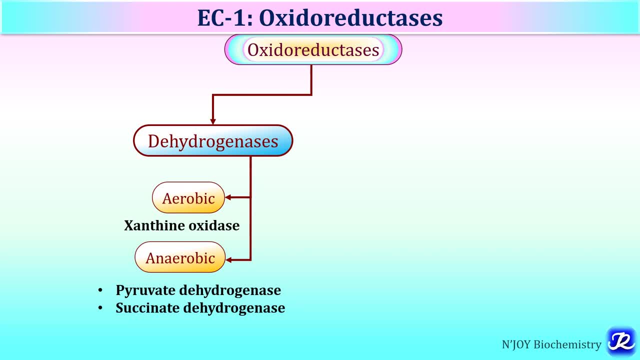 They are called as anaerobic dehydrogenases, for example pyruvate dehydrogenase, succinate dehydrogenase. Oxidoreductases can be oxidases. They catalyze removal of hydrogen from substrate to form water or hydrogen peroxide. Here oxygen is the hydrogen acceptor. The examples are: 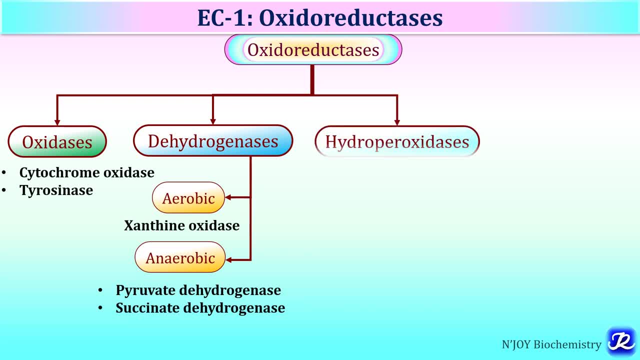 cytochrome oxidases, tyrosinase Hydroperoxidases are also oxidoreductases. They use hydrogen peroxide or organic peroxide as substrate. The examples are peroxidases and catalyses, for example glutathione peroxidase. 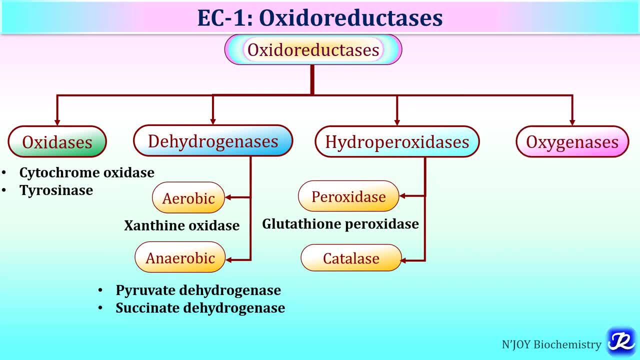 The fourth type is oxygenases. They catalyze direct transfer and incorporation of oxygen into substrate. They can be mono oxygenase, for example phenylalanine, hydroxylase, and dioxyanase, for example homogentisate oxidase. 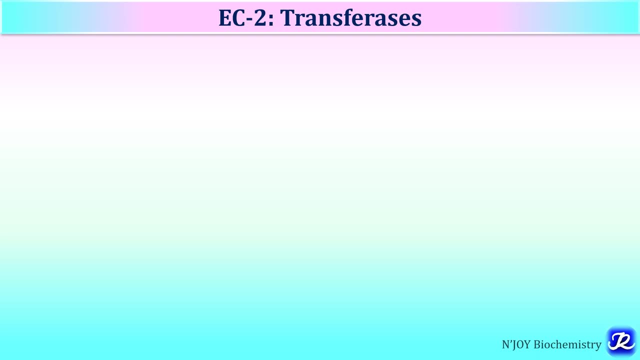 EC2 includes transferases. Transferases catalyzes the transfer of group other than the hydrogen from substrate to another substrate. So which are those other groups, for example, amino group, carboxyl group, methyl group or phosphate group, or any aldehyde group or ketone group? 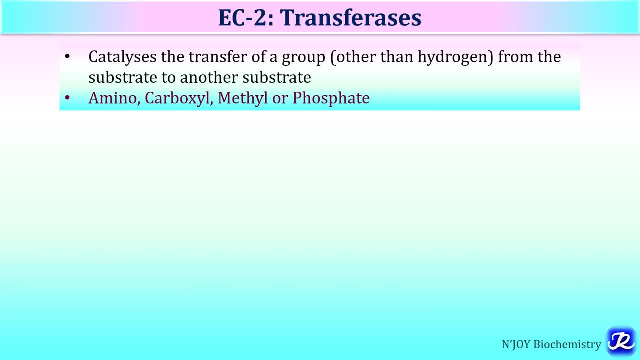 So there is a transfer of group from one substrate to another substrate and this is catalyzed by the enzymes, transferases, which belong to EC2.. So this is transferases. So this is represented as AR plus B, which leads to formation of A plus BR. 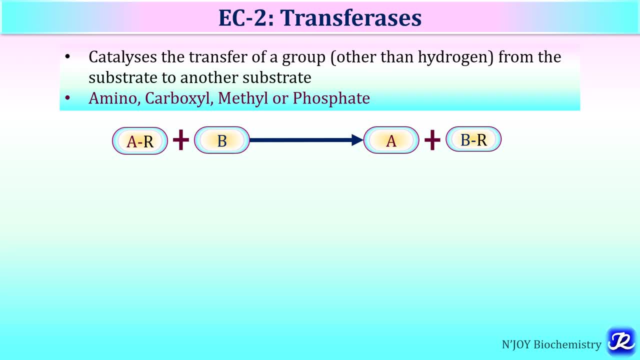 So R is the functional group here which is transferred from A to B to form BR. So, for example, the phosphate from ATP is transferred to hexose, that is B to form ADP and hexose 6-phosphate. So here the phosphate group is transferred from ATP to hexose and this reaction is catalyzed. 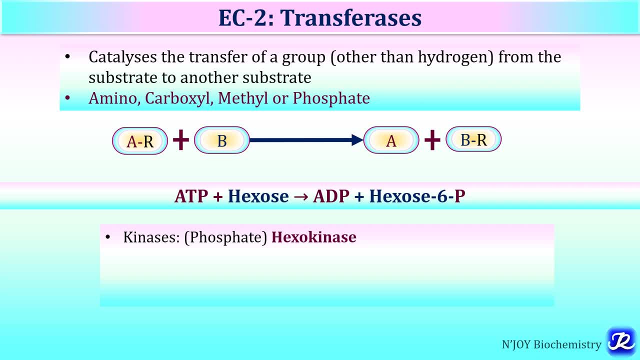 by the enzyme hexokinase, which belongs to kinases, and they transfer phosphate group. The other examples are aminotransferases, or they are also called as transaminases, which transfer amino group from one amino acid to keto acid to form new amino acid and keto. 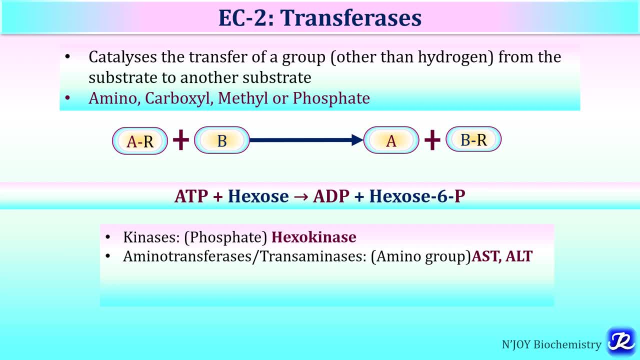 acid, and the examples are aspartate transaminases and alanine transaminases. Trans methylases: they transfer methyl group. Trans methylases: they transfer amino group. Trans aldolases: they transfer aldehyde group. and trans ketolases: they transfer ketone group. 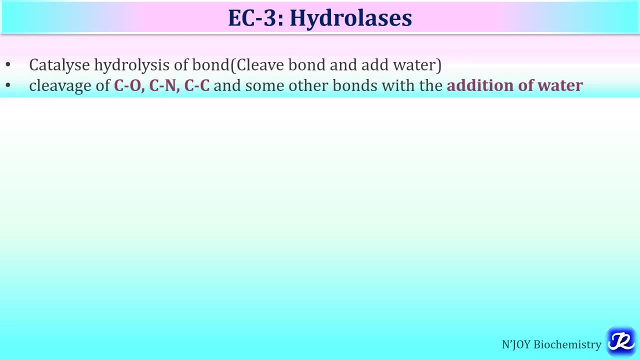 EC3 includes hydrolyses, So they catalyze hydrolysis of bond. Hydrolysis means breaking the bond with addition of water, So they cleave the bond and add water. There is cleavage of bond between carbon and oxygen, carbon nitrogen and carbon carbon. 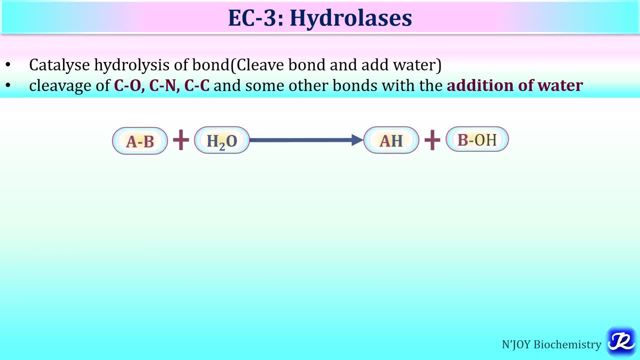 and some other bonds with the addition of water, For example AB plus H2O, which leads to formation of AH plus BOH. All digestive enzymes. they are hydrolyses, For example peptidases. Peptidases hydrolyze peptide bond. 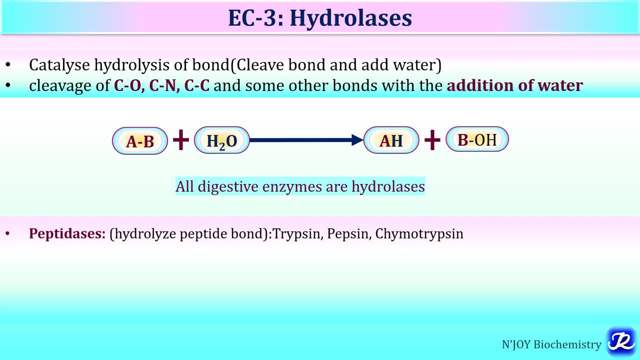 For example, trypsin, pepsin, chymotrypsin- these all are digestive enzymes. Amylase: Amylase hydrolyze the glycosidic bond of carbohydrates. Exonuclease- Exonuclease. 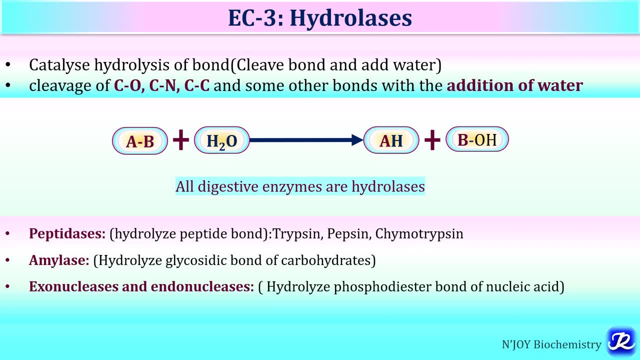 Peptidases and endonucleases: they hydrolyze the phosphodiester bond of nucleic acid. Esterases and lipases: they hydrolyze ester bonds of lipids. So all these enzymes, they are hydrolyses which belong to EC3.. 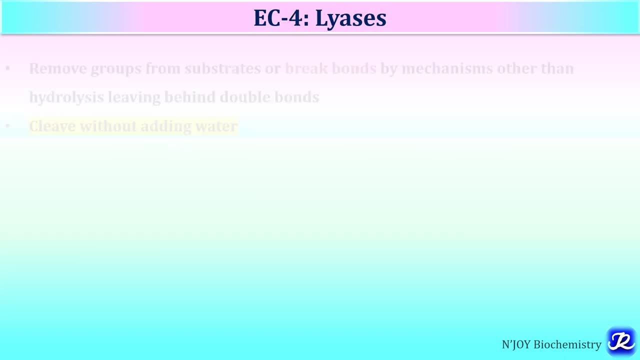 EC4 is lyases, So they remove group from substrate or they break bond. Lyases means breakage of bond, So they break bond by mechanism other than hydrolysis, leaving behind double bond. So hydrolyses they break the bond with addition of water, while the lyases they break the bond. 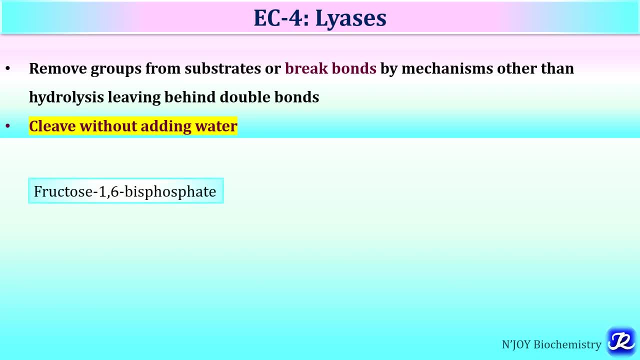 without addition of water, For example, Fructose 1,6-bisphosphate is cleaved to form glyceraldehyde 3-phosphate and dihydroxyacetone phosphate. So this is important reaction in glycolysis, which is catalyzed by the enzyme aldolase. 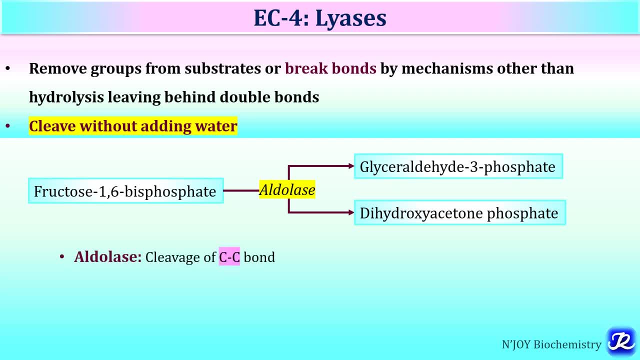 which is a lyase. So aldolase, Aldolase, Aldolase of carbon-carbon bond. Another example is fumarase, which is responsible for breaking carbon-oxygen bond. Arginosuccinate lies, which is the important enzyme in urea cycle, and it is 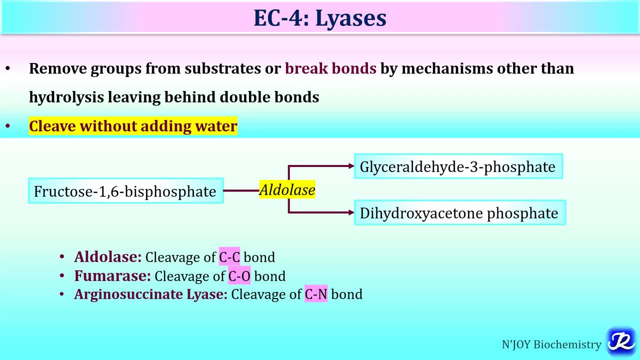 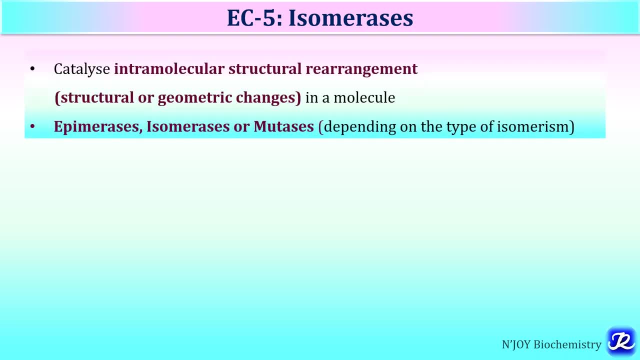 responsible for cleavage of carbon-nitrogen bond EC5 is isomerases. Isomerases catalyze intramolecular structural rearrangement, that is, structural or geometric changes in a molecule, and they are also called as epimerases, isomerases or mutages, depending on the type of isomerism. 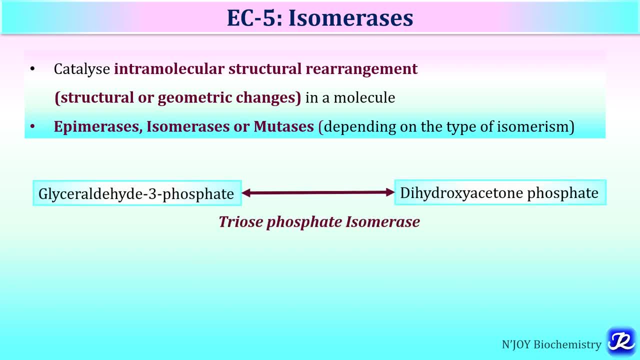 involved, For example, glyceraldehyde 3-phosphate and dihydroxyacetone phosphate. these are the intermediates of glycolysis and they are interconvertible by the action of enzyme triose phosphate isomerases, which belong to EC5.. D-methylmalonyl-CoA and L-methylmalonyl-CoA. they are in interconverted by the action of 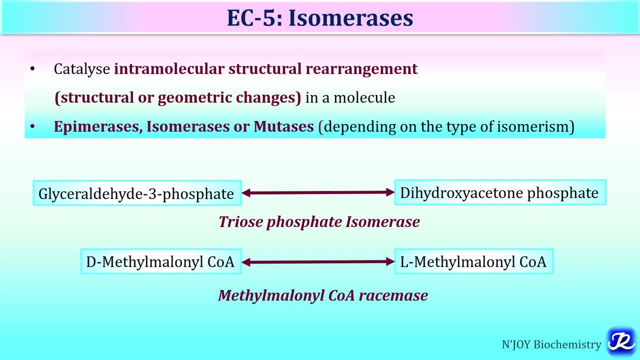 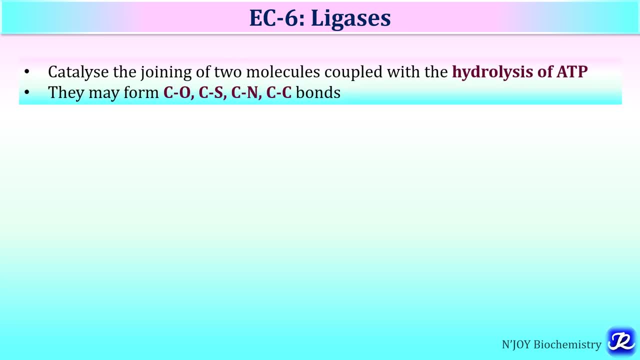 enzyme methylmalonyl-CoA racemase. So these are the example of isomerases. EC6 are ligases. Ligases means they are responsible for joining of two molecules and this reaction is coupled with hydrolysis of ATP. So this reaction requires energy from ATP and there is formation of bond. 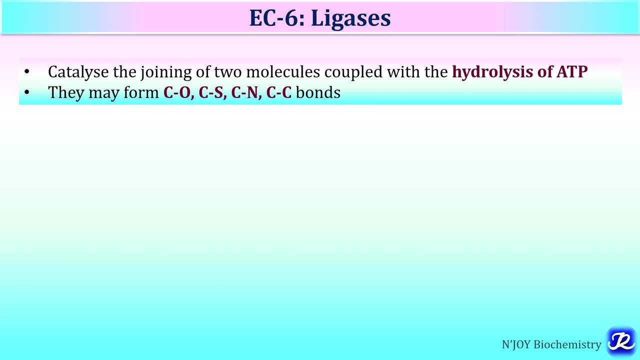 between carbon oxygen, carbon nitrogen and carbon carbon. For example, A plus B plus ATP, which leads to formation of AB plus ADP and inorganic phosphate. The example here is: A represents acetyl-CoA, B represents carbon dioxide plus ATP, which leads to formation. 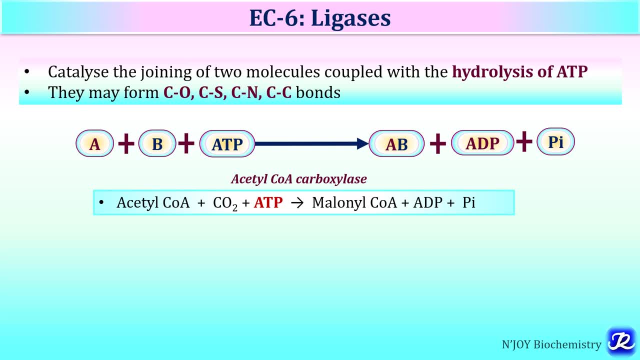 of malonyl-CoA, that is, AB plus ADP and inorganic phosphate, and this reaction is catalyzed by aminoacrylic AA and B inorganic phosphate. that leads to formation of THC. There are multipleホ-Ca responses and these will be represented on the screen first. 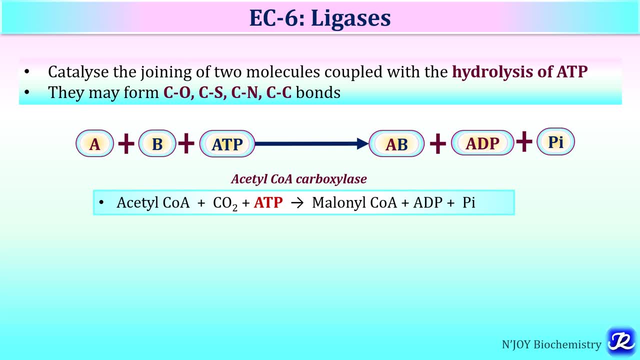 The Basics to Look Out for As an Acetyl-CoA carboxylase reaction. Acetyl-CoA is athren pelicلف Agency and ST serum 97れてv line gee and a longest biobe of carbon and oxygen bond Glutamine synthetase responsible for formation of carbon nitrogen. 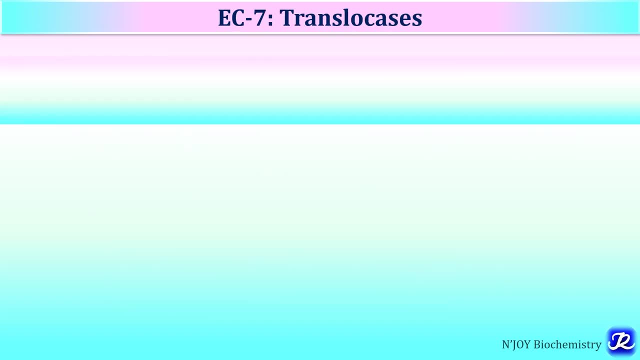 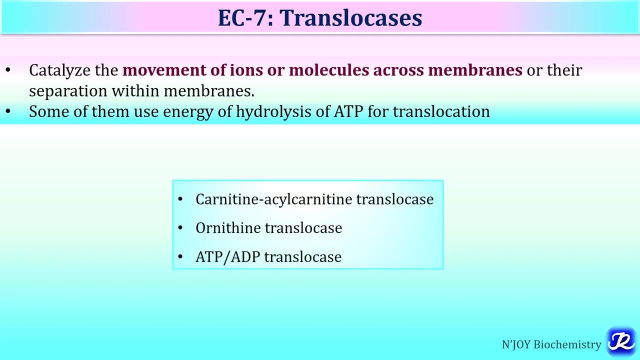 bond EC7 includes translocases. They catalyze the movement of ions or molecules across membranes or their separation within molecules. Some of them use energy of hydrolysis of ATP for translocation. The examples are carnitine, acylcarnitine, translocase and this carnitine. 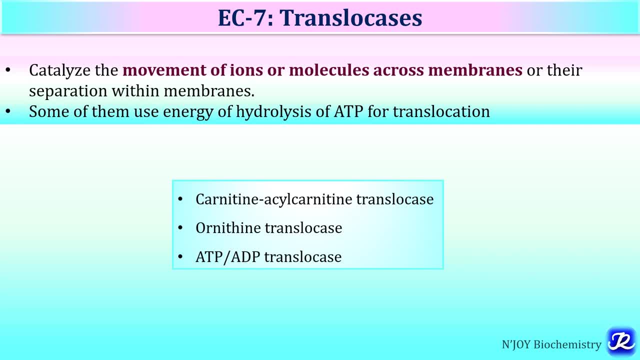 is required for transport of fatty acid from cytosol into the mitochondria for beta oxidation of fatty acid, as fatty acid cannot cross the mitochondrial membrane. Ornithine translocase and ATP, ADP translocases: they are the other examples of translocases which belong to EC7. 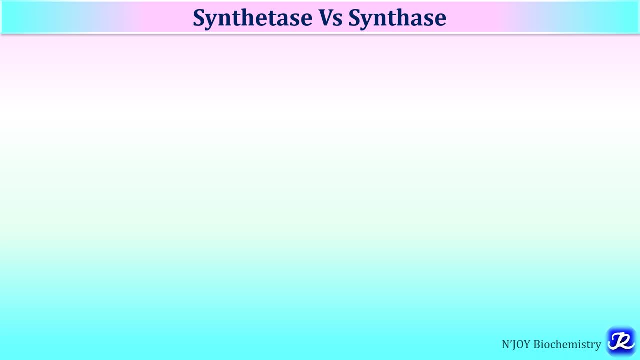 These two terms are repeatedly used in the enzymes, like synthetases and synthesis. So what is the difference between synthetase and synthetase? Synthetases are ATP dependent enzymes which belong to class 6, that is, ligases, For example. 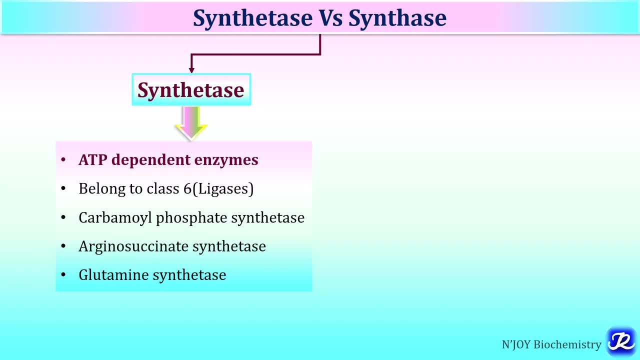 carbamoyl phosphate synthetase, arginosuccinate synthetase, glutamine synthetase Synthase. they do not require ATP directly. They belong to classes other than ligases. They catalyze biosynthetic reactions, for example, glycogen synthase. for the synthesis of glycogen Allosynthase. 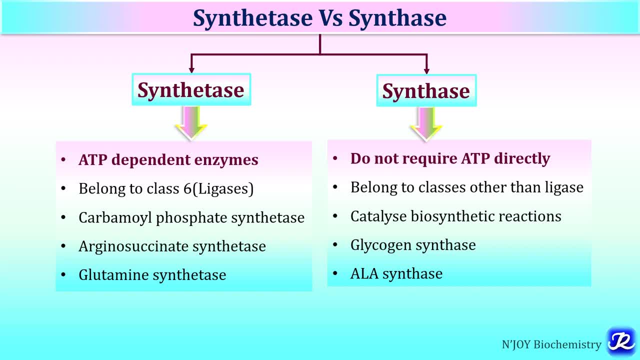 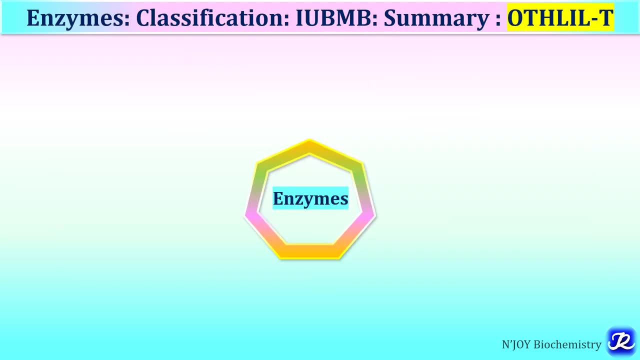 which is used in the synthesis of Heme. So this is the difference between synthetase and synthase. Synthetase T. so this is dependent on ATP and synthase it does not require ATP directly. Now let's summarize today's topic, that is, enzymes definition and its classification. 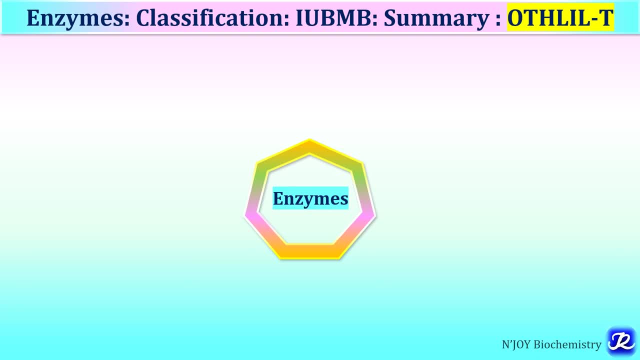 Enzymes are specialized protein produced by living cells that catalyze biological reactions. They convert substrate into product. They are highly specific for their substrate. they are heat labile, water soluble. They accelerate specific chemical reactions without being consumed in the process. The enzymes are classified by International Union of Biochemistry. 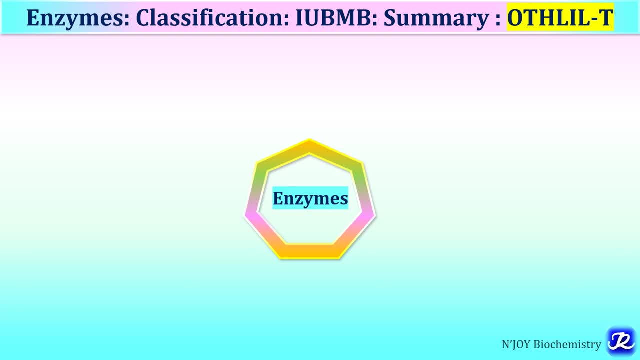 and Molecular Biology and each enzyme has EC number, that is enzyme commission number. There are seven major classes of enzymes which can be remembered as mnemonic orthlyl T. The O represents first EC1, that is class 1, oxidoreductases which transfer hydrogen. 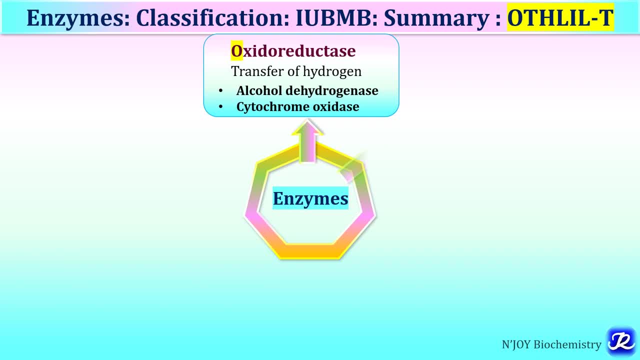 The examples are: alcohol dehydrogenase, cytochrome oxidase. T represents transferases. They transfer groups other than hydrogen, for example hexokinase, alanine transaminases. H represents hydrolyses. They break bonds by addition of water, for example lipases, amylases.